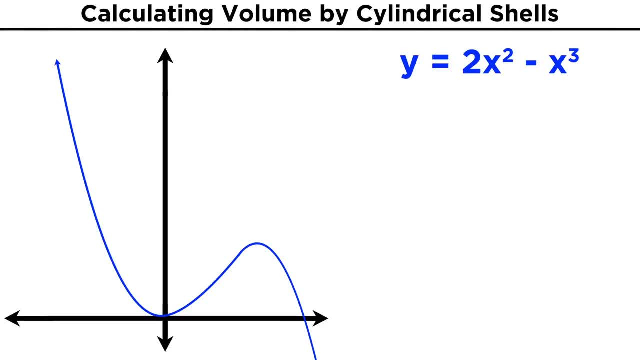 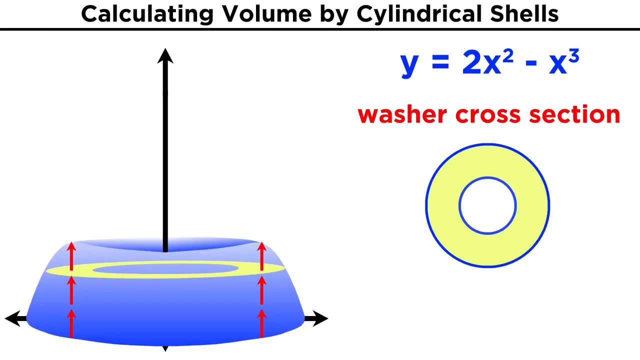 Take for example Y equals two X squared minus X cubed. The region between this function and the X axis looks like this. Let's say we rotate this area around the Y axis to get this bunt cake looking thing, a solid of revolution. A cross-section of this solid would be a washer, given the empty middle region, which we can then push upwards from the base to the top of the solid. But the problem is this. 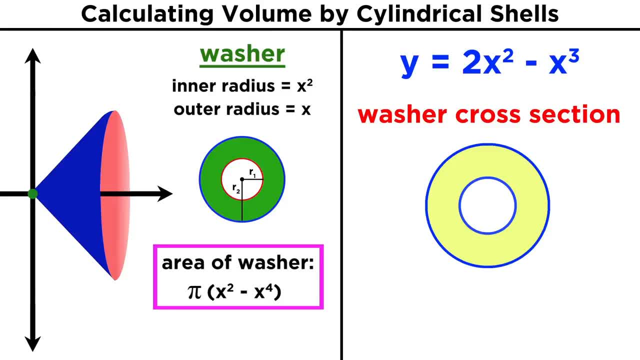 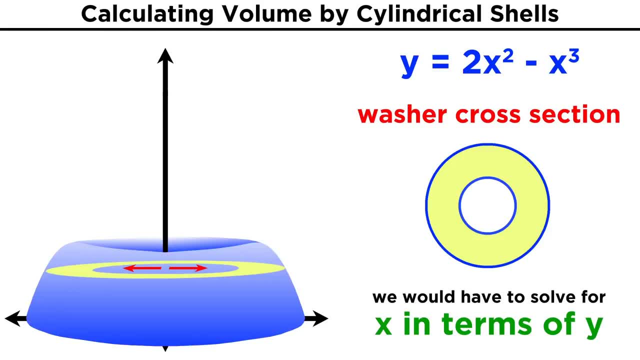 When we did this before, the functions were simple, like Y equals X, or Y equals X squared. Instead of doing these things in terms of Y, with the previous method, we would have to rewrite the functions in terms of Y so that we can integrate. 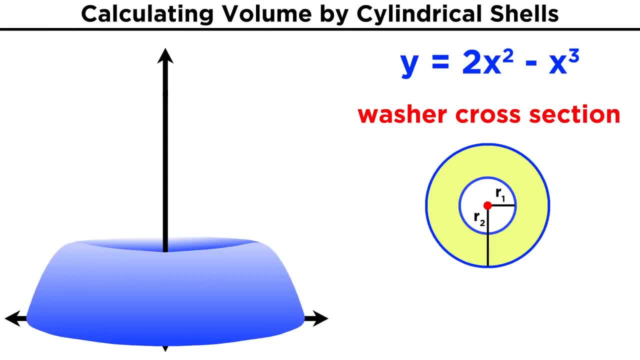 With the other examples, that ended up being no problem, and we were able to get expressions for the inner and outer radii of the washer, that we could integrate. 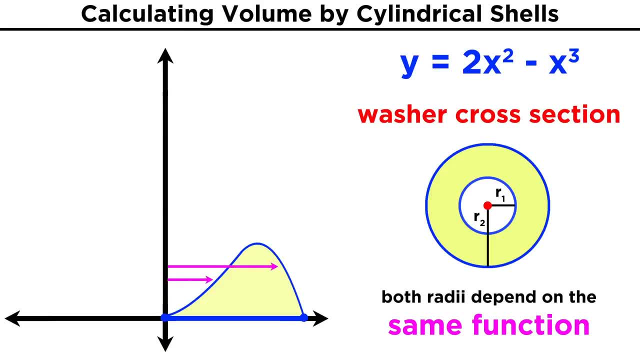 Here it's not so easy. Rather than one function per radius, here both the radii depend on this same function, and furthermore, solving this function for X in terms of Y is not a very appealing task. Let's look at another example. 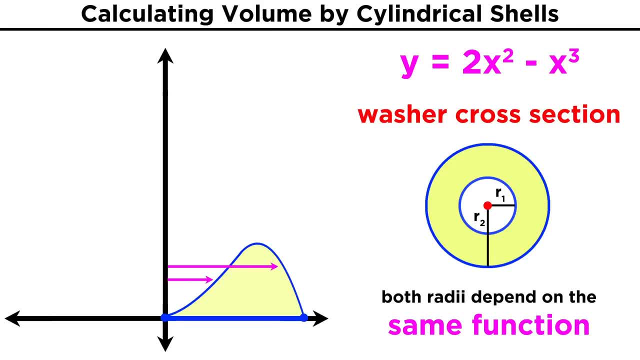 But there is another technique we can try, and it is called the method of cylindrical shells. 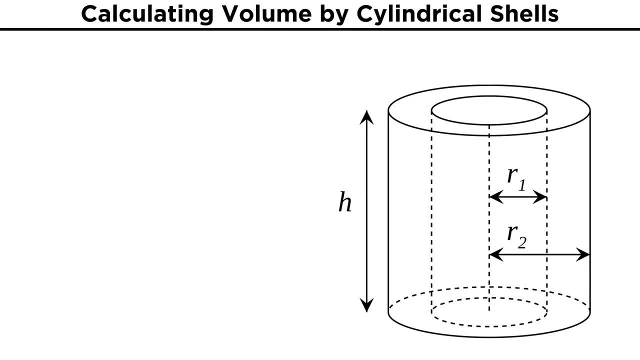 Before we apply this to the problem at hand, let's just look at this hollow cylinder. 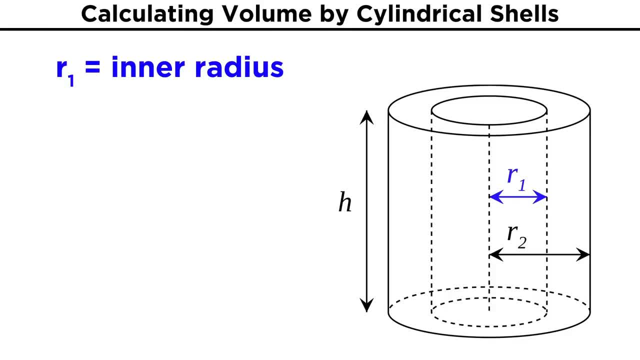 This has an inner radius, R one, which ends at the inner face of the solid, and an outer radius, R two, which ends at the outer face. 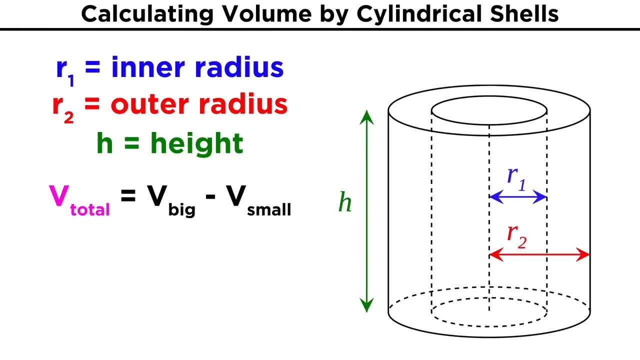 This cylinder also has a height, H. To get the volume of this figure, we can calculate the volume of the cylinder. 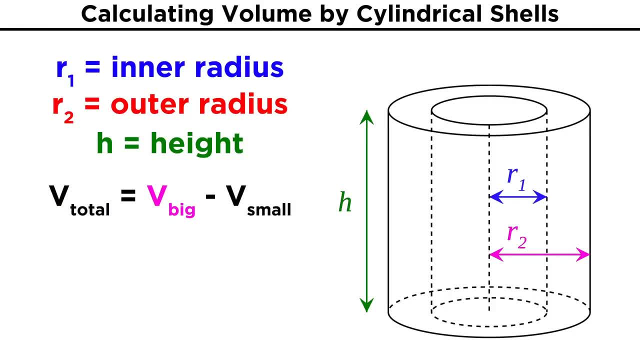 Using R two, pretending that it is solid all the way through, and then subtract from that the volume of the inner cylinder, using R one, since that's all empty space. The formula for the volume of a cylinder is pi R squared H, so let's do pi R two squared H minus pi R one squared H. Factoring out pi and H, we can turn this into pi times the quantity R two squared minus pi R one squared H. This is the volume of the cylinder, and we can use this formula to calculate the volume of the cylinder. 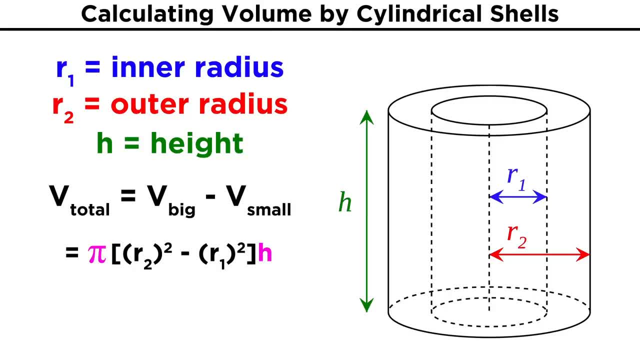 If we remember how to expand a difference of squared terms from algebra, this term is 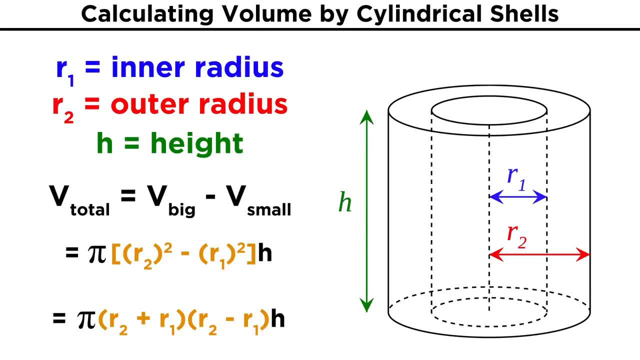 equal to the quantity R two plus R one, times the quantity of R two minus R one. Here's the clever bit. 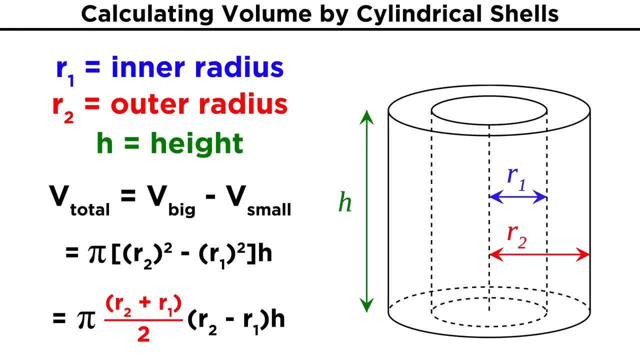 Let's take this sum and turn it into an expression for the average value for the radius. To do that, we just divide by two. But in order to keep the same value, we just divide by two. But in order to keep the same value, we just divide by two. But in order to keep the same value for the equation, let's put a two at the front. Since this is now the average radius, let's just call it R. Then over here, the difference 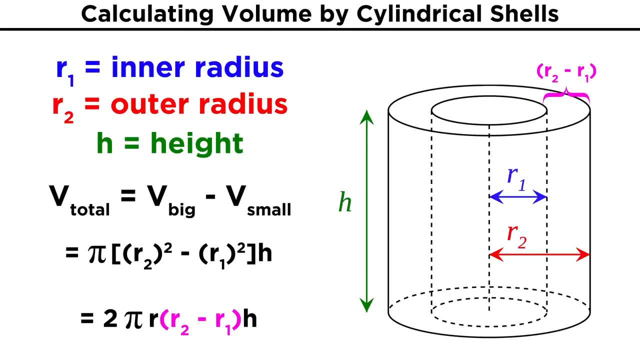 between the radii gives us the thickness of the cylinder, so we can call that delta R if we like. 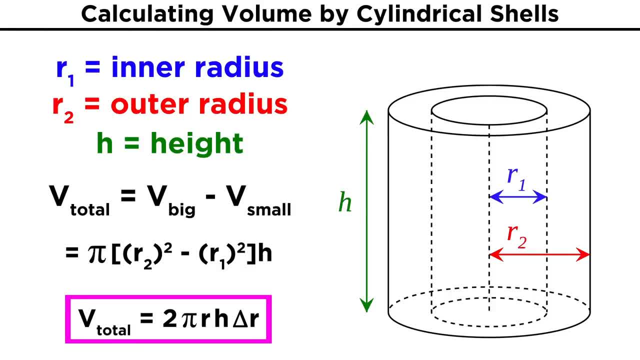 And like that, the volume of this cylindrical shell will be equal to two pi R H delta R. One easy way to remember this is to see that two pi R is the same as the circumference of the cylinder, so this is really just circumference times height times thickness. 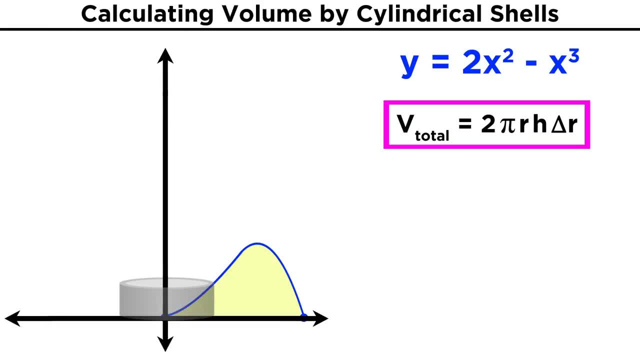 The reason this is useful is that we no longer have to solve for X in terms of Y. If we picture one possible cylindrical shell, it will have a height that is equal to the function F of X, and a circumference equal to two pi X. 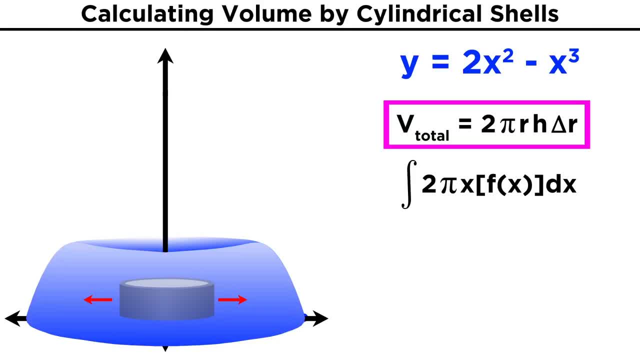 As this shell spans the volume, we then simply have to integrate two pi X times F of X DX. In this case, F of X is two X squared minus X cubed, as we said, so let's plug that in for F of X. 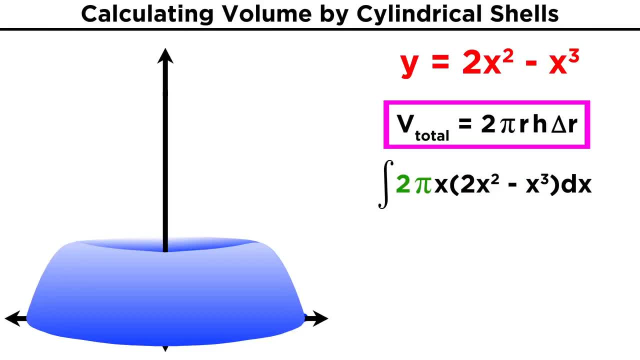 And then to simplify, we can take two pi out of the integral, but the X must stay, and it can be distributed across the other term. That leaves us with two pi times the integral of two X squared minus X cubed. That leaves us with two pi times the integral of two X squared minus X cubed. 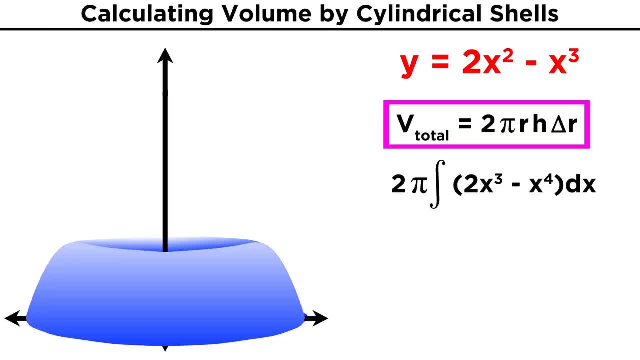 That leaves us with two pi times the integral of two X cubed minus X to the fourth, DX, evaluated from zero to two. 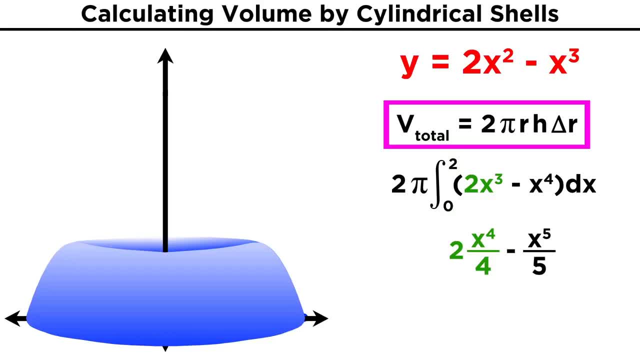 We integrate to get two X to the fourth over four, or one half X to the fourth minus one fifth X to the fifth. 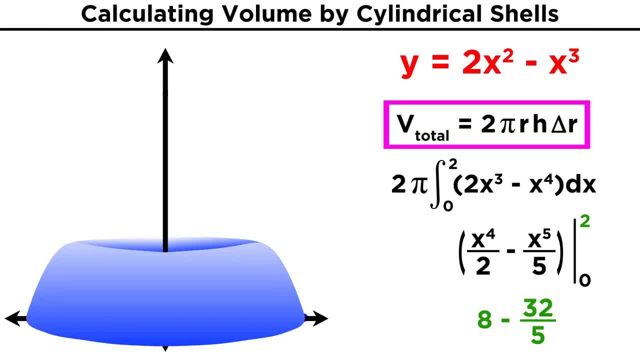 We evaluate at two, and we get eight minus thirty-two fifths, or forty minus thirty-two over five, so we subtract and multiply by two pi 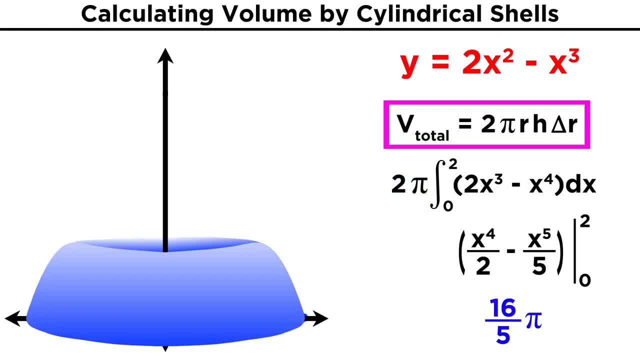 to get sixteen fifths pi. 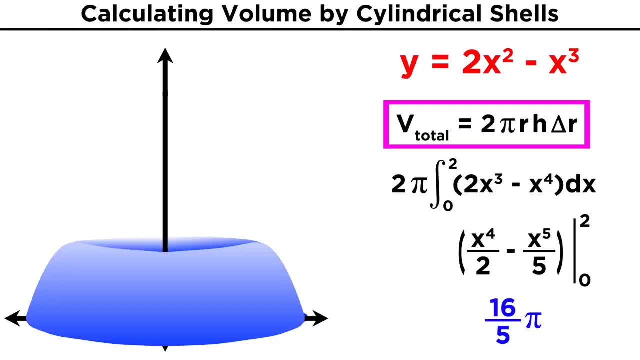 So while this may have seemed complex, part of that is because we derived the formula 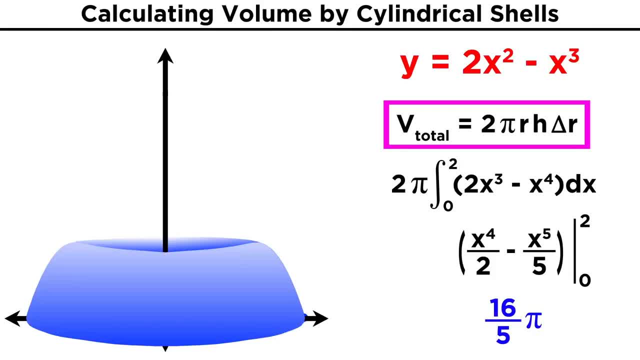 for the volume of the cylinder. We won't have to do that every time, we just need to know that the volume of the solid with a cylindrical shell oriented vertically will be equal to the integral of two pi X times F of X DX, over the interval that spans the solid. 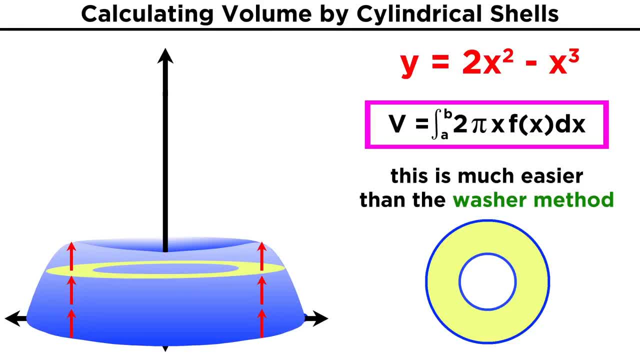 So we can see that for this particular example, this method ended up being easier than the washer method we used in the previous tutorial, as our formula for the volume of the cylindrical shell was ready to go, which meant we didn't have to do much to set things up. 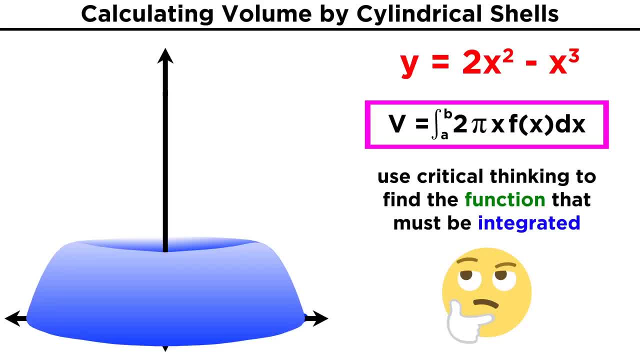 For any solid of revolution you are looking at, whether the cross section is a disk or washer, you will just have to think critically to figure out which approach is best, depending on whether it is easy to find the right solution. 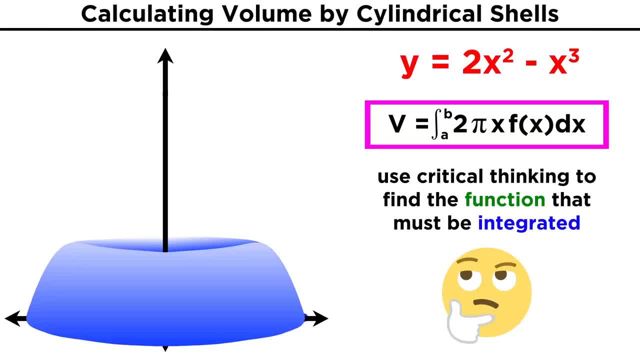 So we can see that for this particular example, this method ended up being easier than the radius or radii of the cross section with the function or functions as given, or whether it is easier to express things another way. 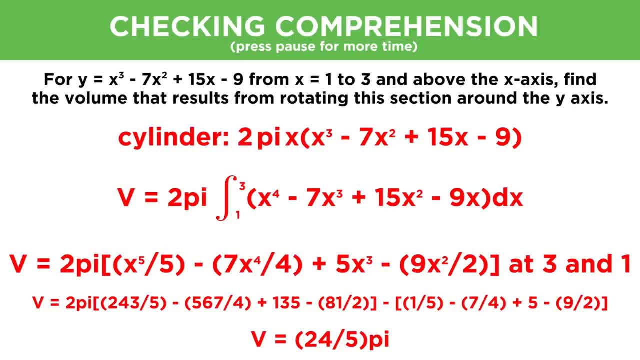 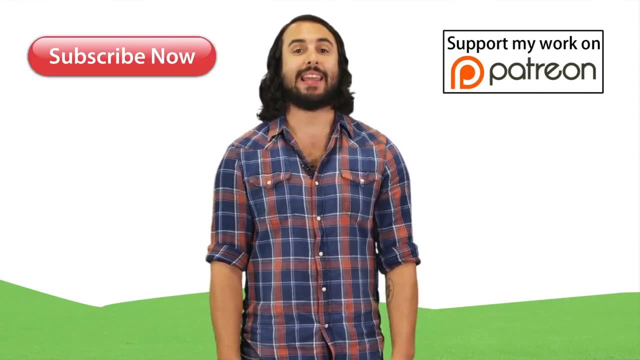 Thanks for watching guys, subscribe to my channel for more tutorials, support me on patreon so I can keep making content, and as always, feel free to email me, professordaveexplains at gmail dot com. 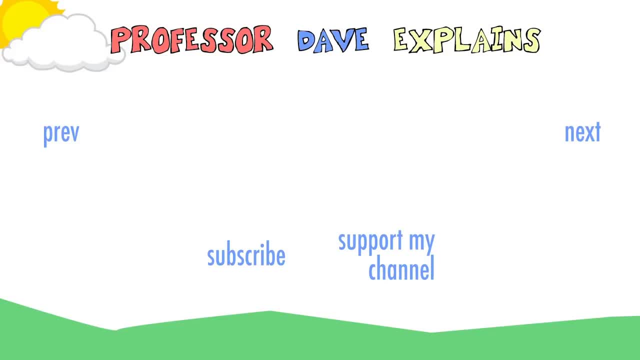 I'll see you next time, bye! Beautiful machine. 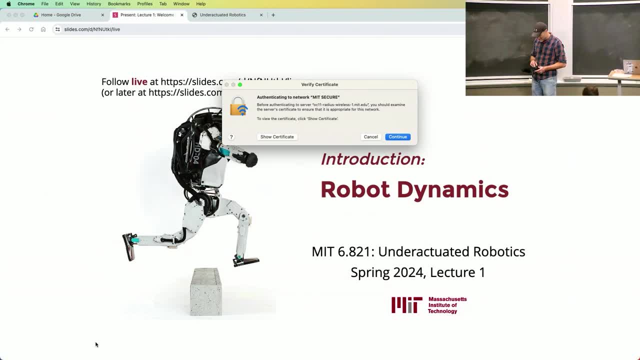 That was going to go badly.